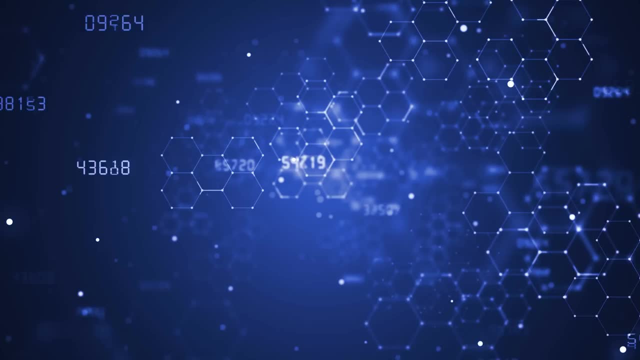 How long do you think it would take you to find the adjustment? Say I'll get the meu ad reduce spoken valor000 of against adlist promise also states that just programming at least a few hours, unless you get really lucky, That's the power of. 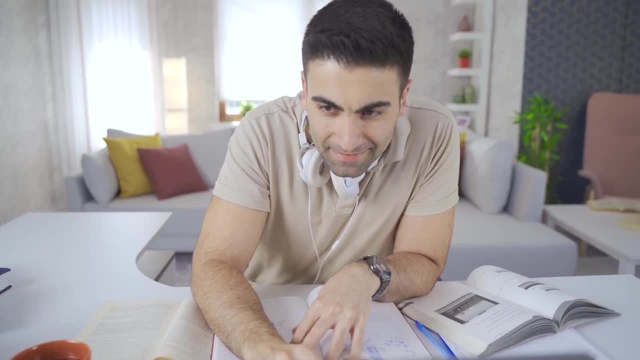 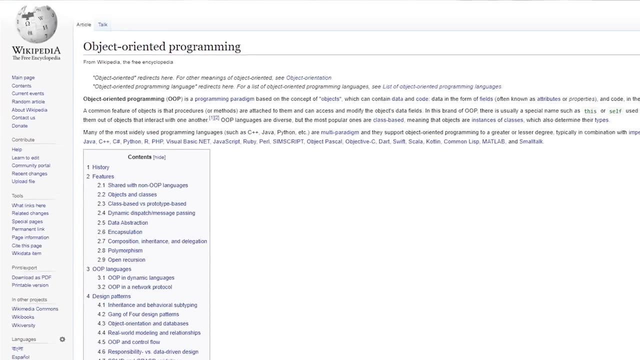 data structures. I hope that this example makes you even more excited about learning data structures and algorithms. To make learning DSA easier for you, I recommend that you learn at least one object-oriented programming language before you start DSA. That's because most online resources on DSA will be using an. 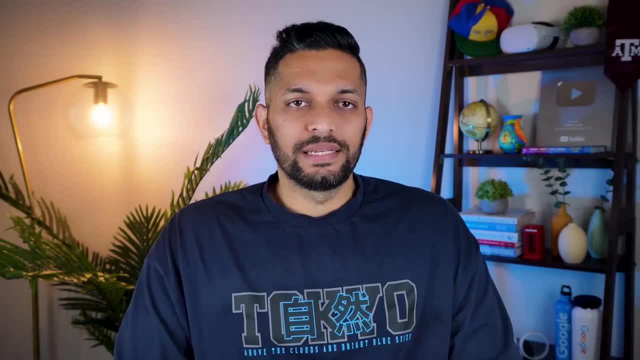 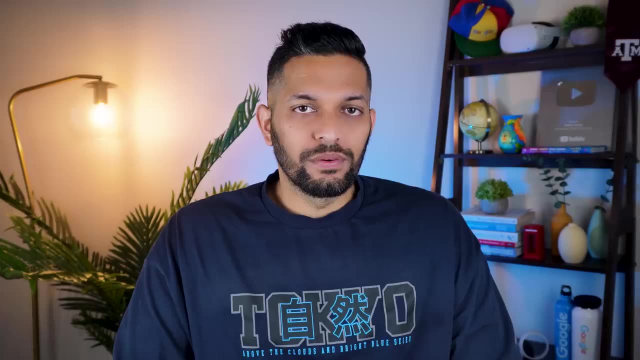 object-oriented programming language. You can pick any popular language like Java, JavaScript, C++ or Python. If you already have a language you are comfortable with, you can continue with that, But if you don't, I recommend that you pick Python for DSA. That's because Python is less verbose and you can write code really. 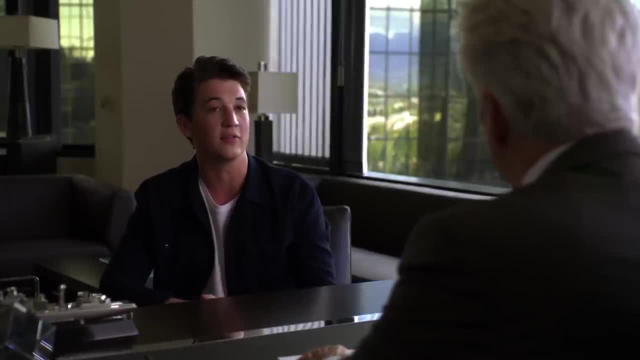 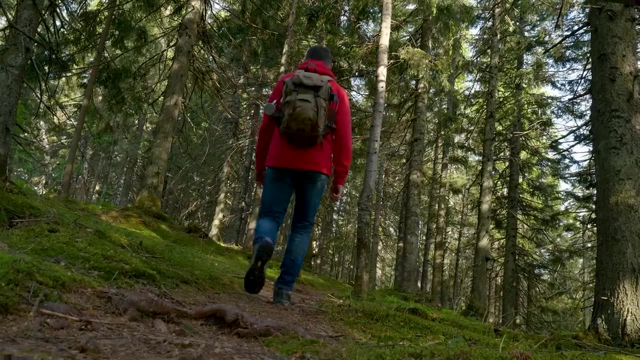 fast in Python And in an interview where you only have 45 minutes to solve a question, this would be really helpful. Now that we have that out of the way, let's talk about how I started my DSA journey. If you have seen any of my 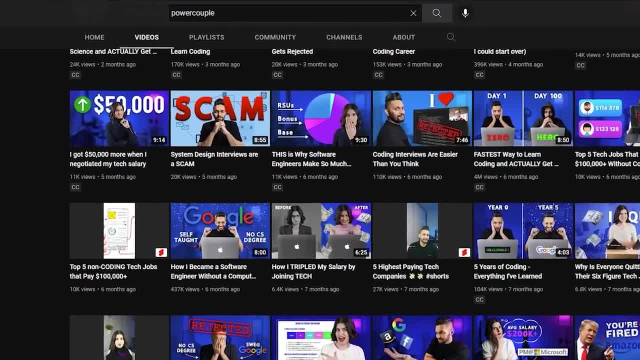 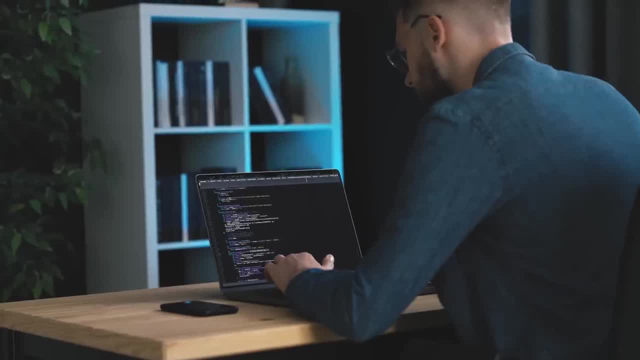 previous videos. you know that I'm a strong advocate for learning by doing. Unfortunately, for DSA, I don't think there is any good resource that you can jump into and start learning by doing. That's because DSA requires a good technical foundation Before you can actually apply it to any. 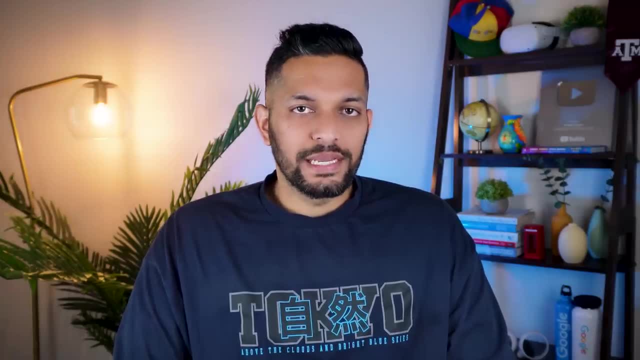 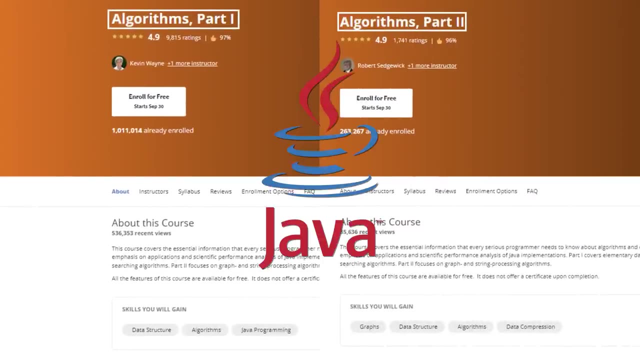 new problems. That's why I took the online course route for DSA. I use this course called Algorithms by Princeton University on Coursera. This course is divided into two parts and is taught in Java, But if you're looking for a good 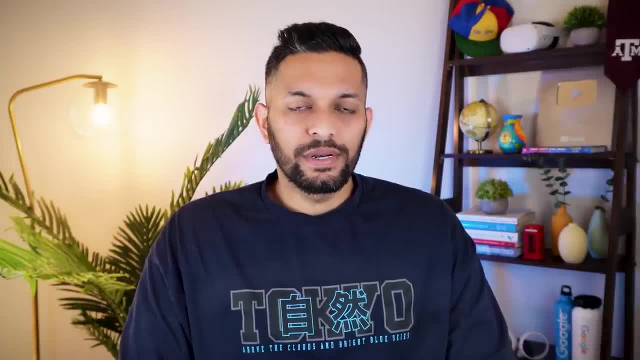 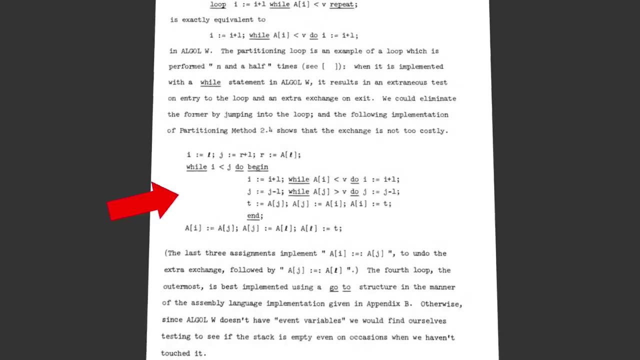 DSA course in languages other than Java. I do have some recommendations for you later in the video. Professor Sedgwick, who is one of the instructors of this course, is famous for taking the worst-case space complexity of Quicksort from Big O of N to Big O of L. 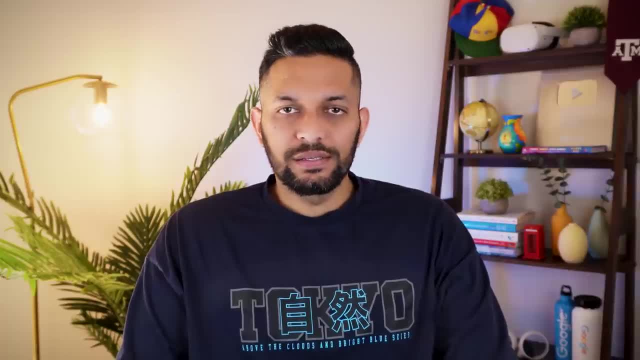 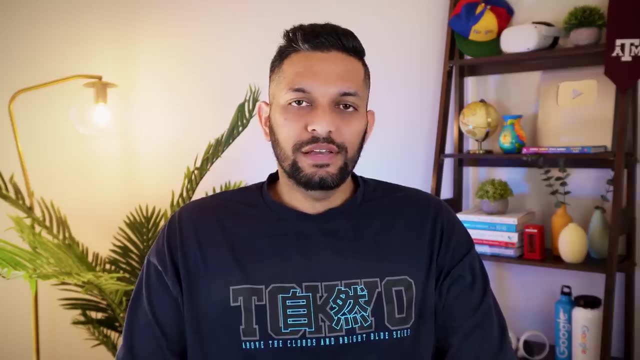 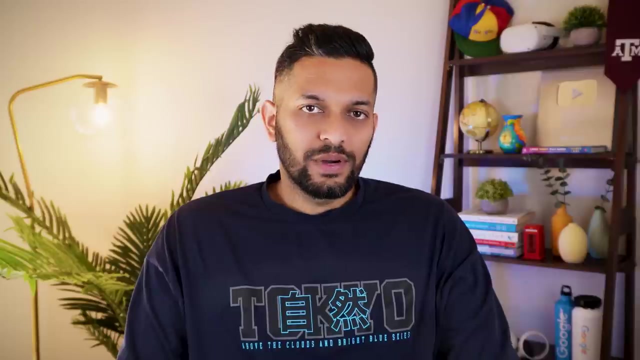 If you don't know what that means, don't worry about it. The point I'm trying to make here is that this course is taught by the best of the best. The instructors of this course have seen many algorithms come and go during their career. Their book on algorithms has been a best-seller since 1980s. That's why. 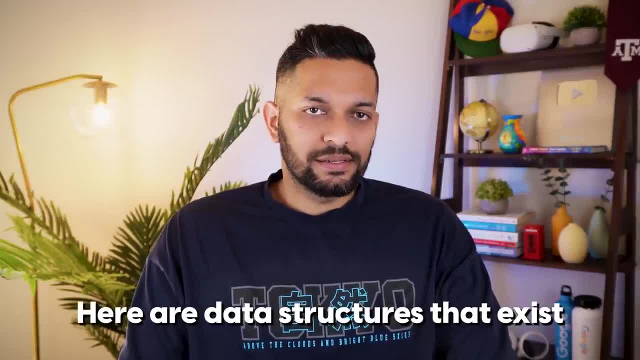 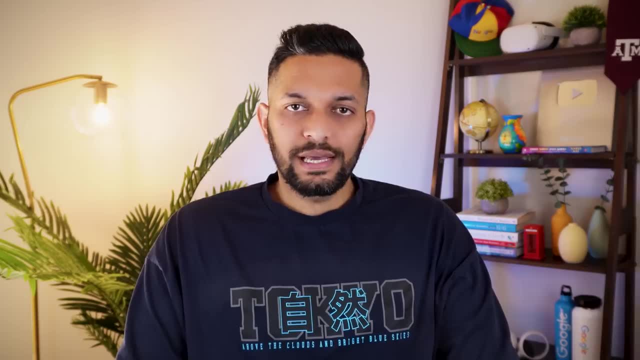 instead of just saying: here are data structures and algorithms that exist. they are able to provide a complete context of why a data structure or algorithm exists and when to use it. And, purely from a learning standpoint, this course will make you feel like you're learning something new. This course will help you. 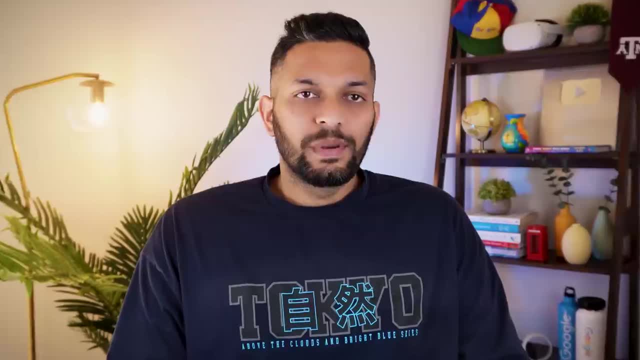 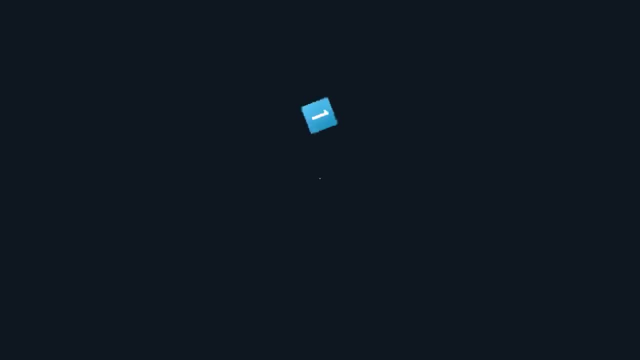 fall in love with algorithms. I cannot recommend this course enough. But there is one big issue when it comes to learning DSA: Most people don't know how much is enough and where to draw the line, And I also made a mistake here. This. 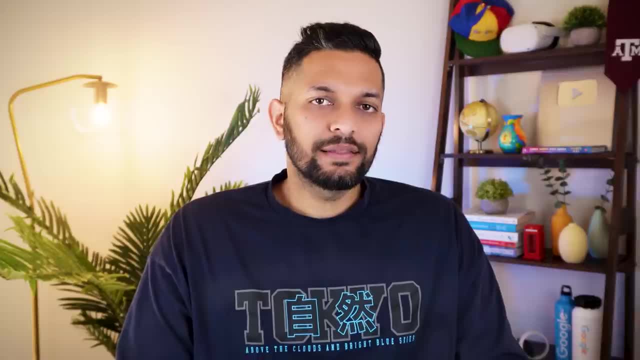 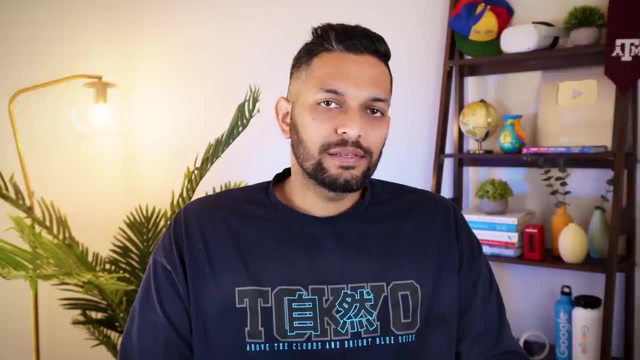 is the first of the three big mistakes I made on my journey. I'll share the other two later in the video. The mistake I made was that I ended up completing both algorithms 1 and algorithms 2.. I realized this much later in my journey that I did. 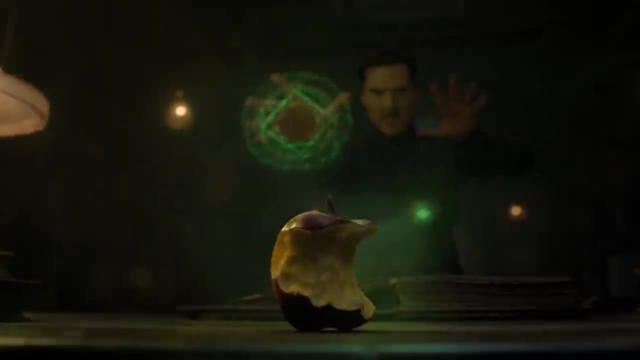 not need full algorithms 2 for coding interviews. If I could go back in time, I would skip the entire week 3 and go back to the beginning of the course. I would skip the week 3 and everything after week 4.. I'm not saying that these things are. 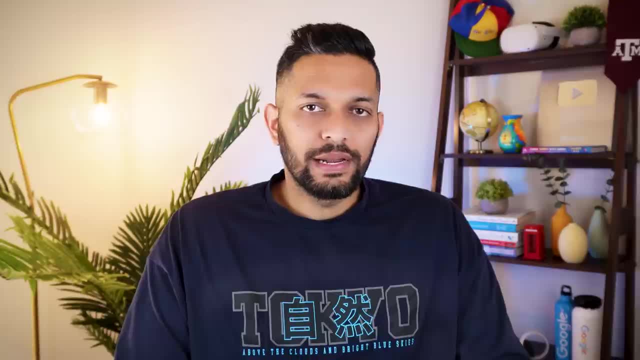 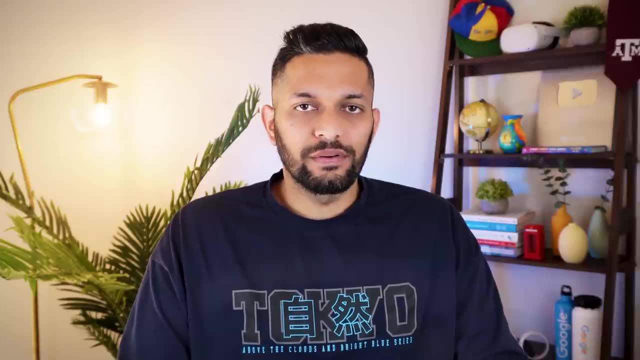 not useful. It's just that they are rarely asked in the interviews, And even if there is some uncommon question that uses them, you would be able to solve it if you follow what we are going to discuss in the rest of the video. Anyway, if Java is not your primary, 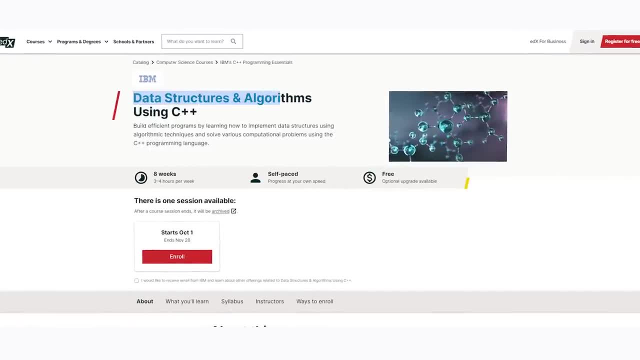 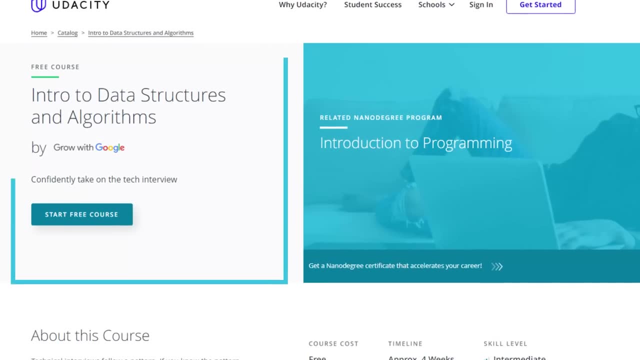 language and you want to use C++ instead, there is this course by IBM that you can use. If Python is your language of choice, you can use this course by Google on Udacity: This Udacity course might not be free in your country, but it's free in the US And you 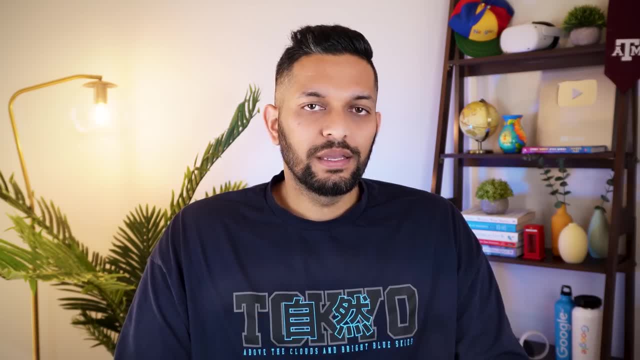 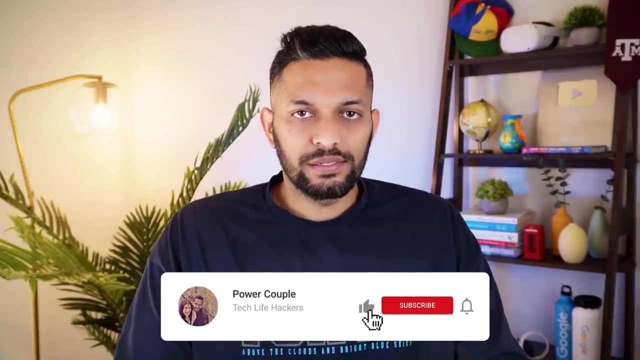 can get it for free in the US. All the links will be in the description. By the way, in case you are wondering, I do not get paid anything if you use any of the resources I am recommending today. So the only way to support us is by subscribing. 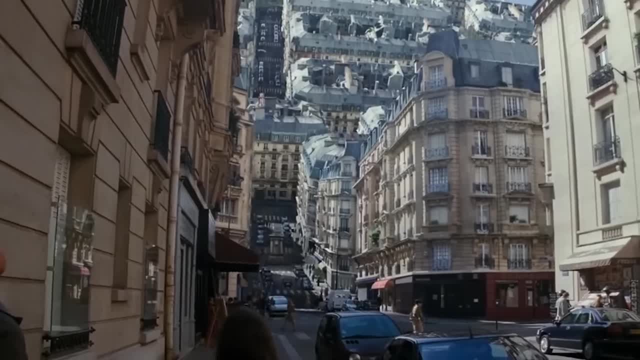 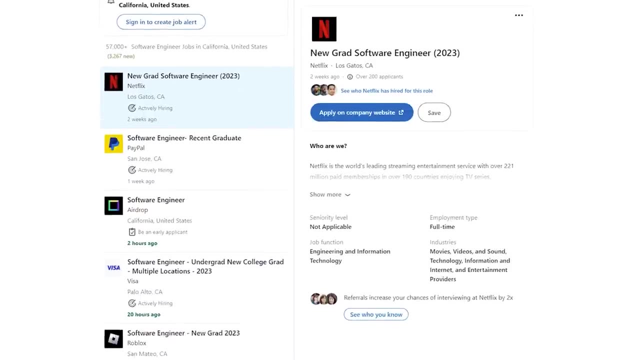 After finishing a course on DSA, you will become very powerful And you might start believing that you can bend the entire universe to get the dream job. And that would be the second big mistake I made. I applied for many jobs after completing DSA, but it did not. 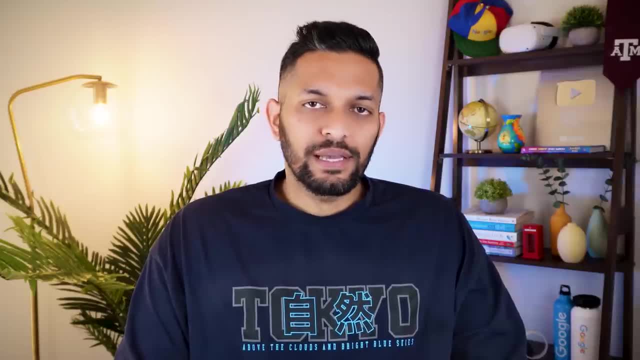 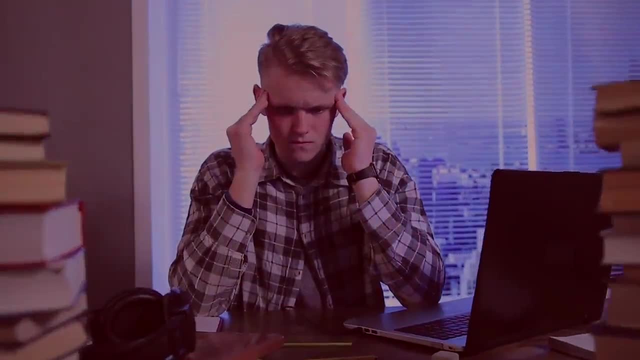 get me anywhere. That's because knowing all these different algorithms and actually applying them to a new problem are two very different things. Add the interview time limit of 45 minutes on top of that and it suddenly starts to look like an impossible task For those. 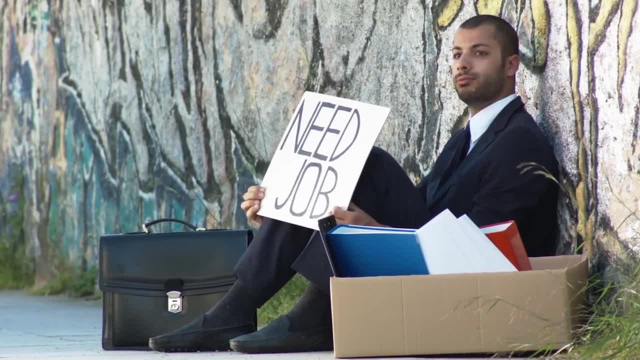 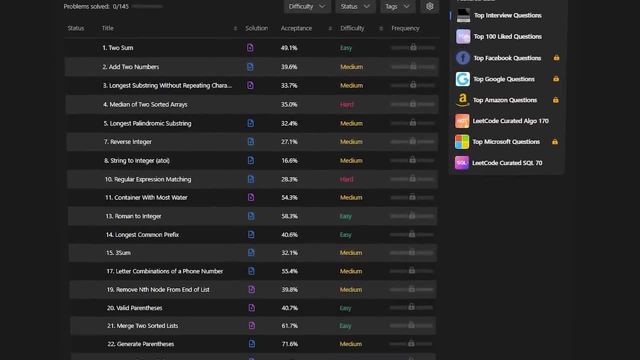 who are having a hard time finding a job, even after learning DSA. trust me, I have been in your place. Here is how I solved that issue. I went to Leetcode and started practicing some interview questions there. If you don't already know, Leetcode is pretty much the best resource. 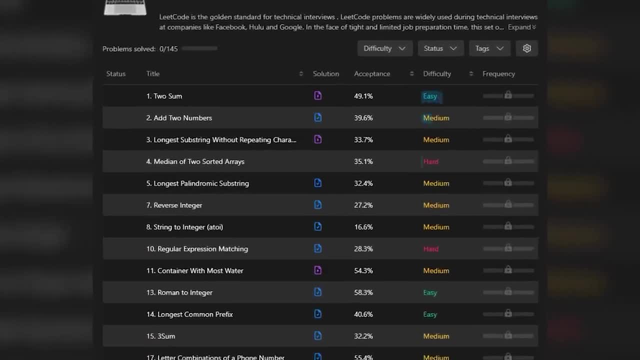 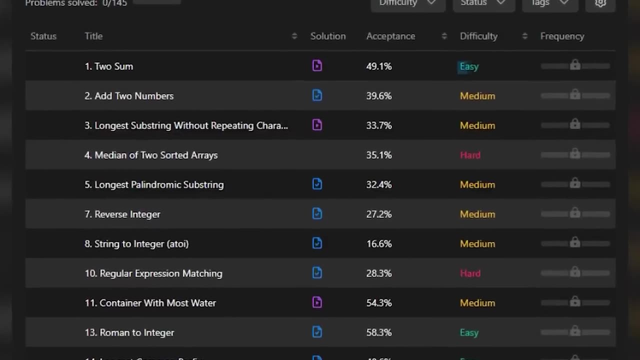 out there to practice DSA questions. All the questions are labelled easy, medium or hard based on the difficulty level. In the beginning you might not know what DSA is, but once you get used to it you will understand. You might not be able to solve medium or hard problems, so stick to the easy.